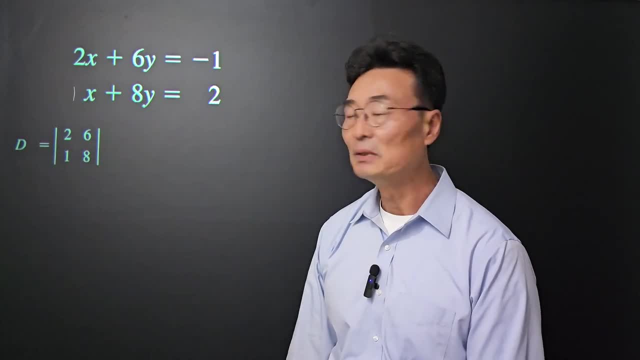 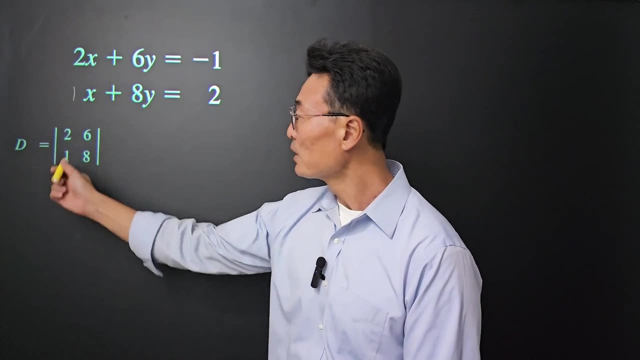 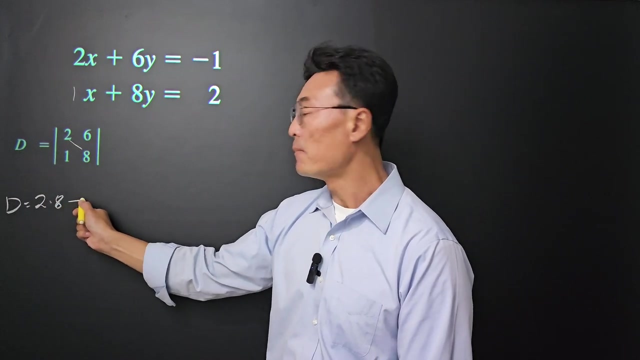 x and y of the second equation. put it in the second row, Next the bars that we have on the left and the right represents the determinant of the matrix, meaning we take the 2 multiplied by 8, so d will equal to 2 times 8 minus the other cross, or 6 times 1.. And if you do this, 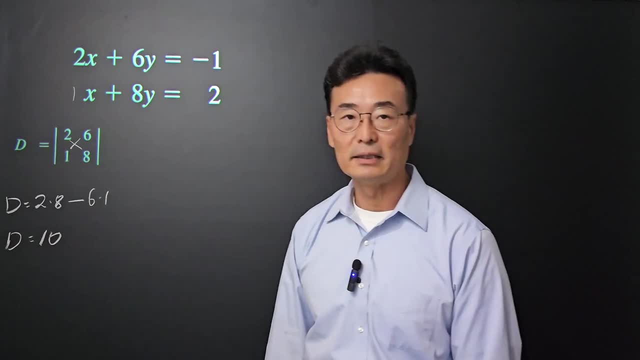 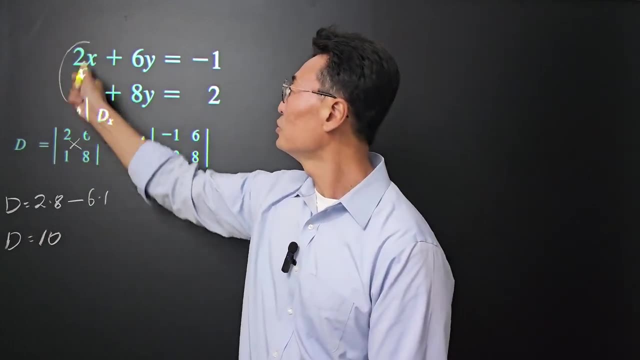 we get d is equal to 10.. Next, we also need to find the dx. What dx is is that we take the 2 and the 1 that we have remove from the first column and instead replace it with the negative. 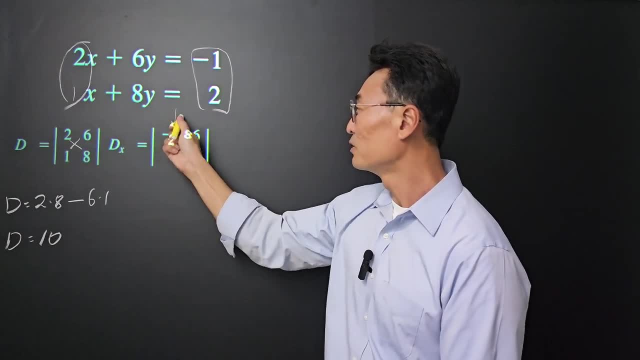 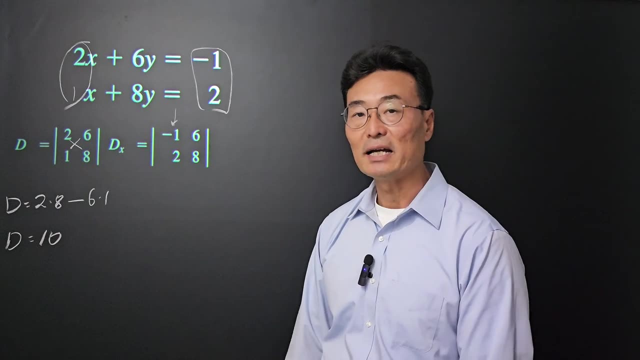 1 and the 2 that we have on the right side of the equal sign, like so in the first column, Notice the second column, the 6 and the 8, we leave it alone, since we're looking for dx, To find dx. 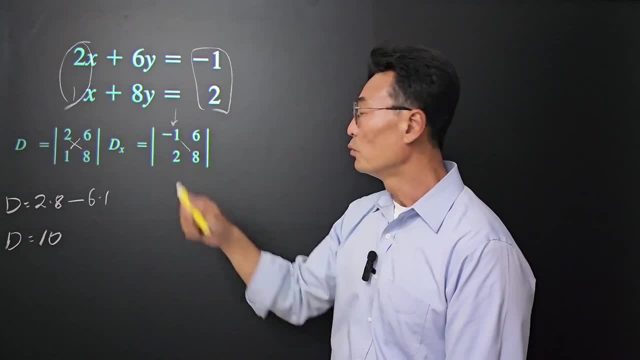 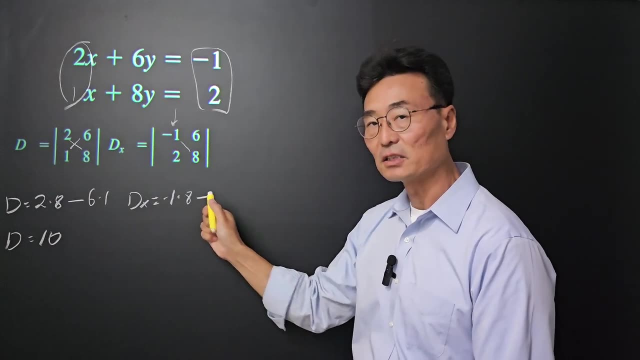 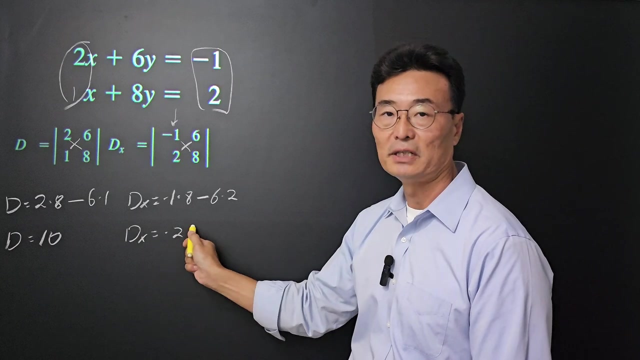 we're finding the determinant of this matrix. or first, we take the negative 1 times 8 minus, it's always minus 6 times 2. And if you do this we get dx is equal to negative 20.. Next, 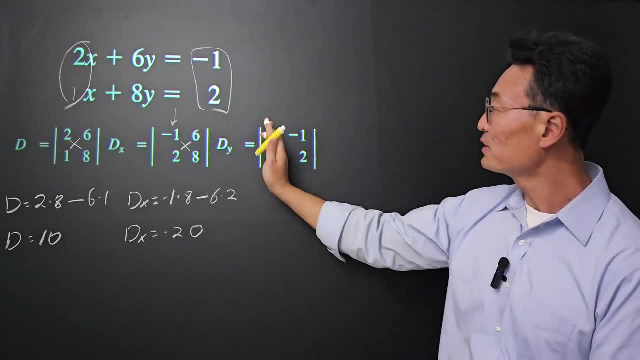 we need to find. dy. dy is leaving the first column alone with the 2 and the 1 that we started with. This time we're going to be removing the 6 and the 8 from the first column and we're going to 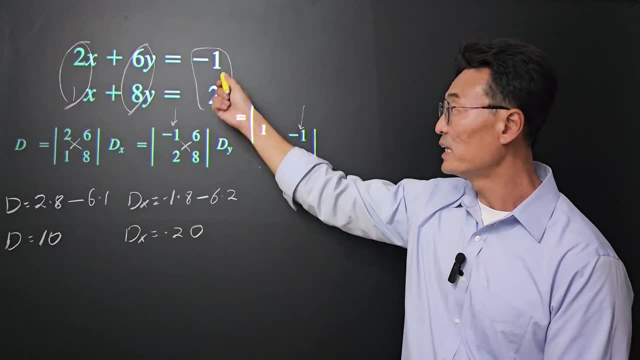 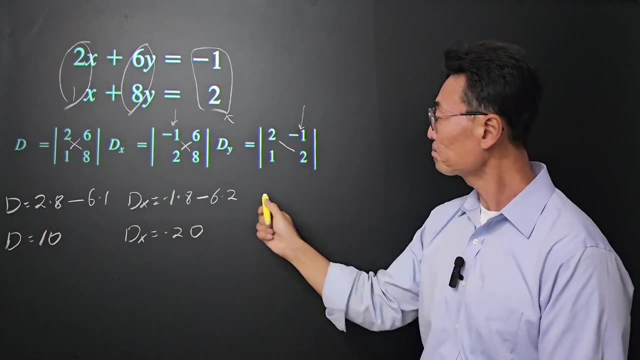 the 8 and plugging in the 1 or the negative 1 and the 2 that we have on the right side of the equal sign. To find the determinant. again, we multiply 2 and the 2.. So dy will be 2 times 2 minus the. 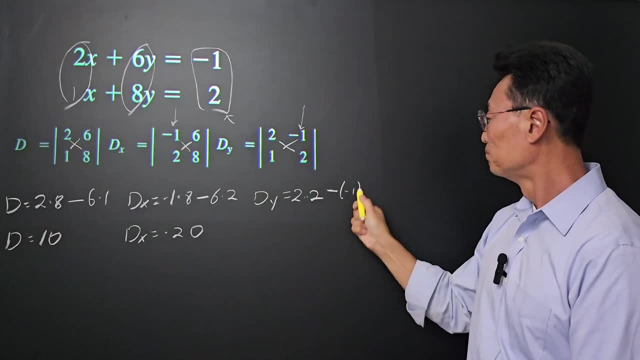 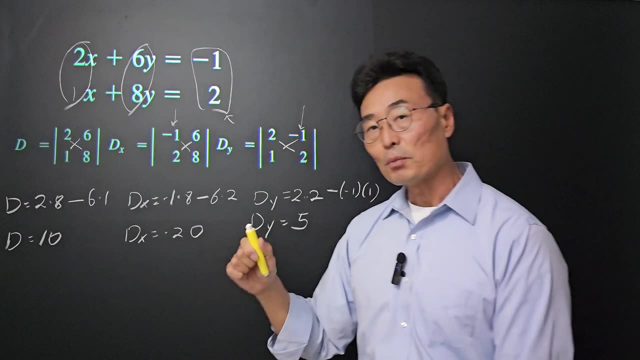 other cross, which will be negative 1 times 1.. Then, if you work this out, we get 5.. We're almost done To find x. what we want to do is we want to find the determinant of this matrix or 6 times. 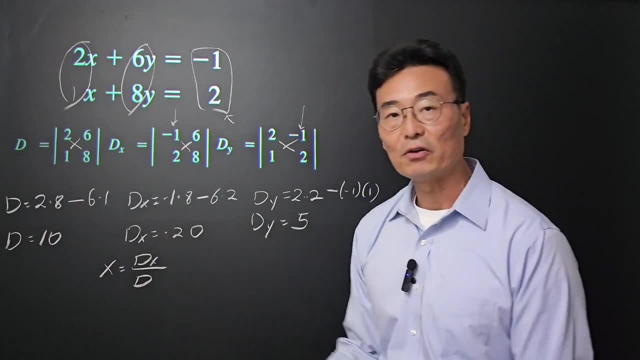 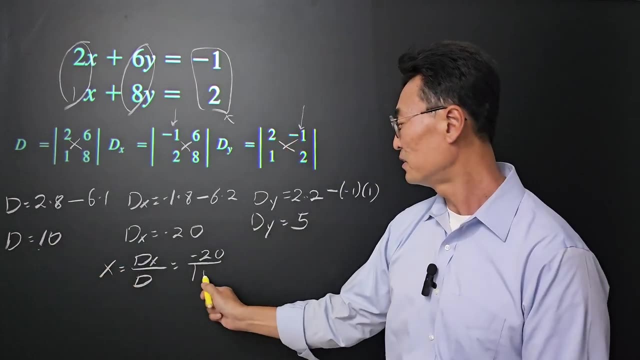 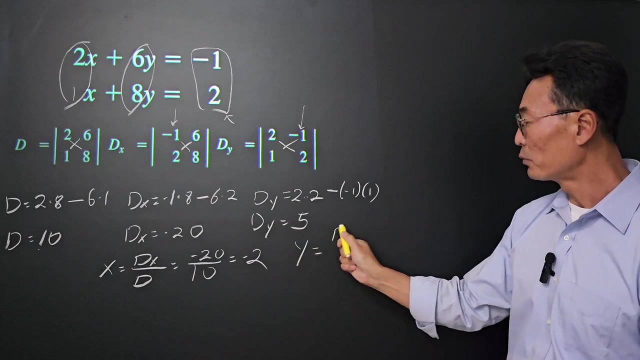 2. We want to do dx over d. that we worked out earlier And dx is negative 20. d was 10 that we have here, So then x will be negative. 2. Also, to find the value of y, we want to do dy over d.